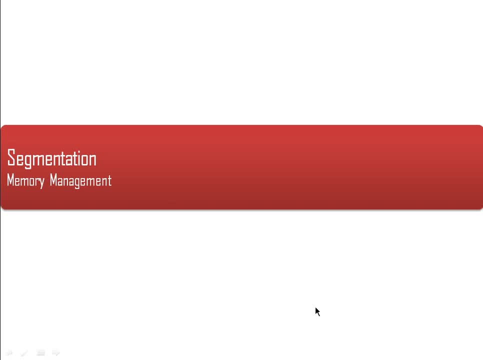 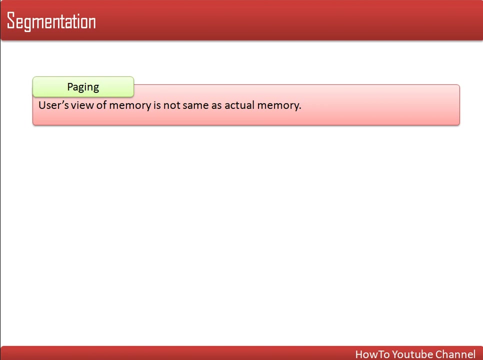 hello everyone. in this video I will explain segmentation in memory management in operating system. so before segmentation we have seen paging technique. so in paging users view of memory is not same as actual memory. you might read this line in your book as well. so what is the meaning of this line? 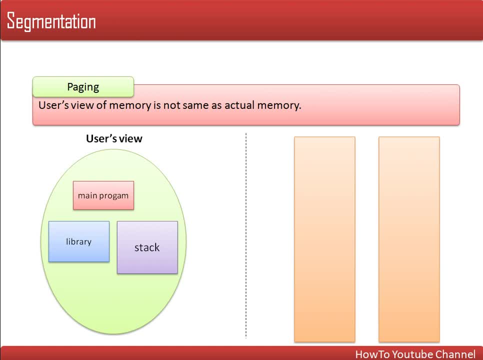 what users think when we execute any program, what we think. that program will be loaded in memory somewhere and library required by that program will be loaded in memory somewhere. so these module are loaded in memory all together. so this is the users perception. but what actually paging does? paging will divide. 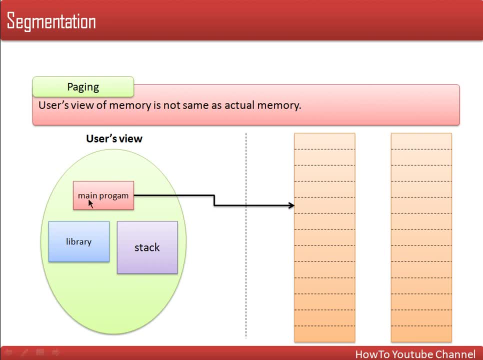 our program into a fixed length of pages and this memory also divided into similar length frames. one page can be loaded in any frame. so user is thinking main program is loaded in memory all together, library is loaded in memory all together and stack area used for stack is in. 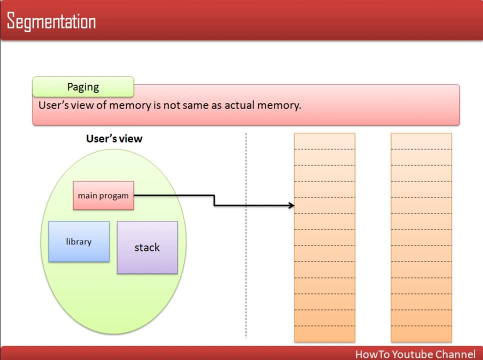 loaded in memory all together but in actual what paging is doing, paging is dividing this main program into multiple pages, and that pages can be stored in any frame. so let's say this main program divided into two frame, as sorry, two pages. one page is stored in this frame, another page is stored here and 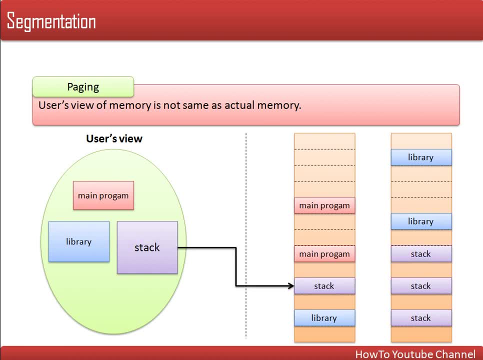 similar for library and for stack. so if you can see, this is the users view. we are thinking our entire program is loaded in memory up at one place but in actual that program is loaded in memory at different print place. so paging actually separate users view from the actual memory. so here comes the rule of 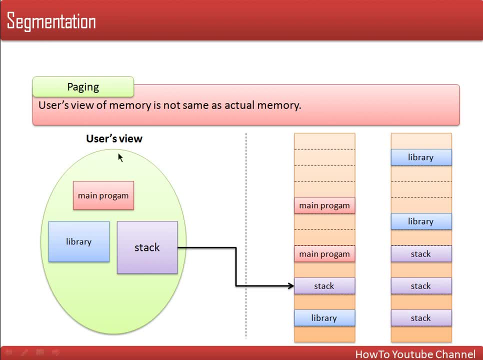 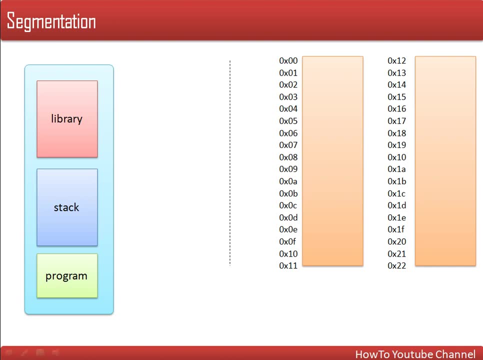 segmentation. segmentation actually support this view. so segmentation says that modules loaded in memory at one place, like library is loaded here, stack loaded somewhere here, here all together and program is loaded here. so this one is actually supporting the users view. user is not concerned with whether the program is loaded in memory before library or after stack, users just. 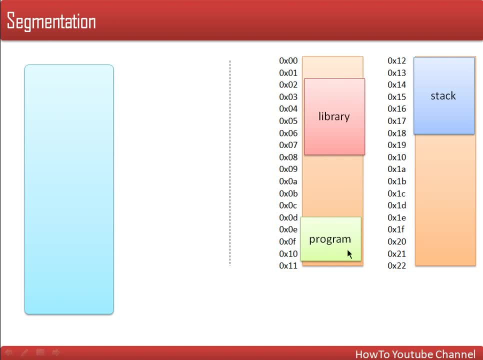 having an idea that our entire program is loaded in memory at one place altogether. segmentation, actually following this approach. now, the thing is that how a element in segmentation is going to be addressed, how address are generated, how those addresses are converted into physical addresses, so every segment actually having a name. 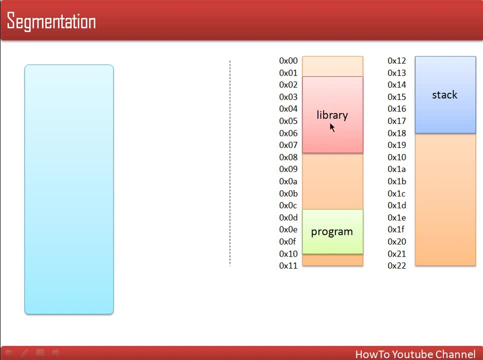 now in this segment if I want to access any particular byte. so what we need to give, we need to give the name of this segment that I want to access- library segment- and in this segment we have to specify offset, like which byte I want to access: second byte, third byte, fourth byte of fifth byte. so information I have. 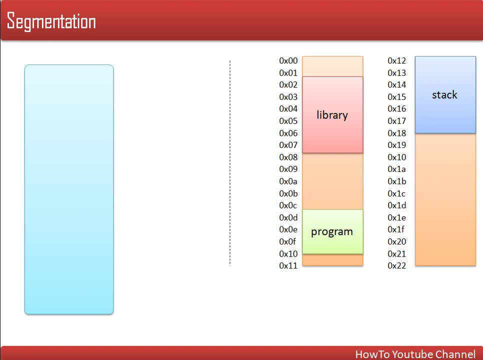 to provide segment name and offset, but for simplicity, instead of taking name, number is assigned for every segment. so these information actually stored in the table. segment number: what is the number of segment? what is the base address like? what is the starting address in physical memory for that? 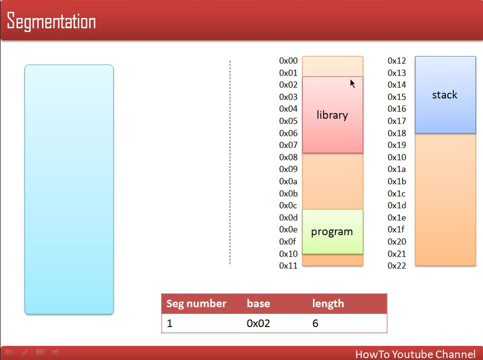 segment and what is the size, what is the length of that segment? so if we look at the library segment, let's say number one, assigned to this segment, the starting address, if you can see this, is the two and the length of this library: one, two, three, four, five, six, six five. these information will be stored in table. so 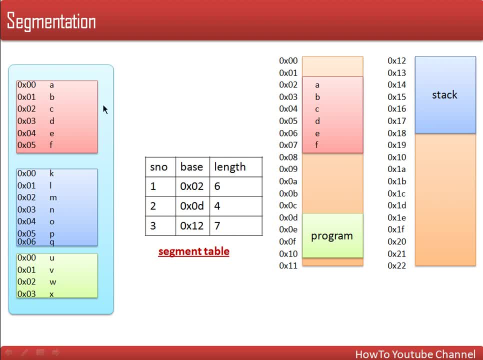 let's have a look on this one. so we are having here three segments. these segment are having some information like ABCD, and this is actually specifying the offset, like: this is the first byte, this is the second, a second, third byte, fourth byte, fifth byte, sixth byte. so in every. 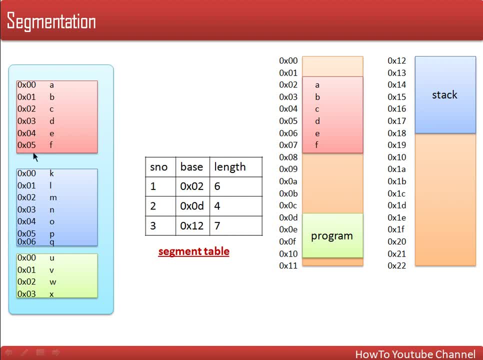 segment. we have shown segments and all segments are stored in memory. so, if you can see, first segment is stored at 0 to base address. second segment, second number we actually given to this one. so second segment is stored at 0, D base address and third one stored at 0, 12. so this actually a hexadecimal representation: 0, X and the 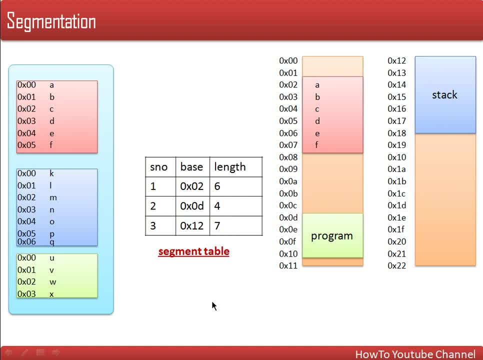 length of first one 6, then 4 and here 7. so if someone want to access a particular byte in segment, some data in segment. so let's say user want to access this element see. so user need to specify to information segment number and the offset. so user has specified that the access data is. 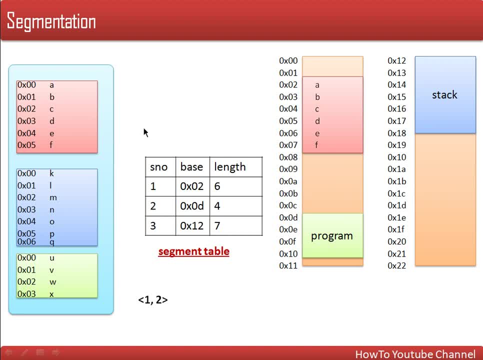 stored at this address. so this address is having segment number one and this is the offset. so whenever this address is specified first of all base address of that segment is first. so this is the segment number. this segment table will be checked so we are having segment one here. this is the base address, so this address will. 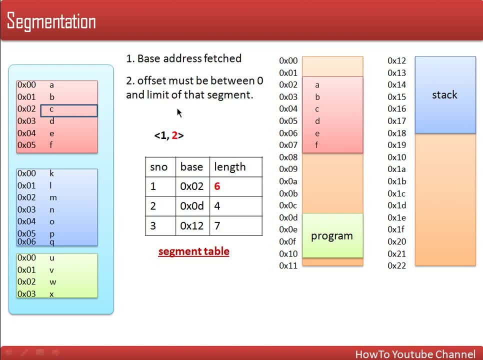 be first. next thing it will be checked that this offset must be between 0 and the length of that segment, like if a user is specifying invalid at is like 1 and 10. so we can see here this segment is having length only 6 byte. so 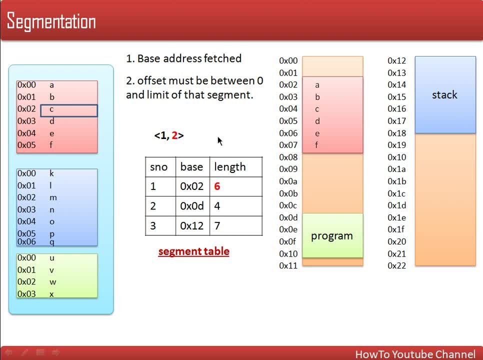 then given 10 in address is invalid. so in that case error will be generated. but here offset is less than this number and greater than 0. so it must be between 0 and limit of segment. so it can be 0 here because we are having our offset is. 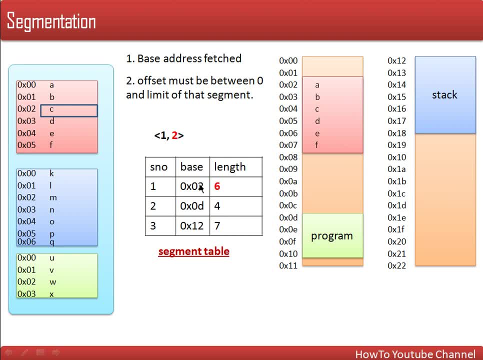 starting from 0. so if this condition is satisfied, in that case we will go for 3 third step. what is the third step? this third step will take this base address and offset will be added in this address. so we are having base address 2, offset will be added. it will give us: 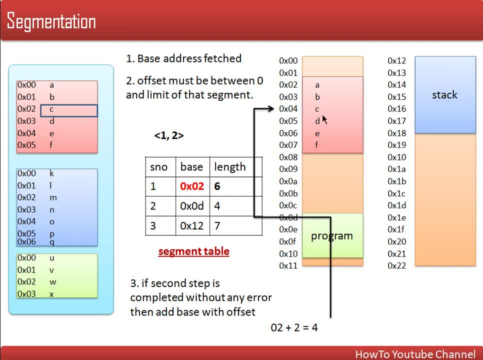 4. we will go to address 4 and we will fetch c. so the process for resolving is: address in segmentation base address will be fetched, offset will be checked whether that offset is a valid offset or not, in case if that is a invalid offset, if that given offset is more.